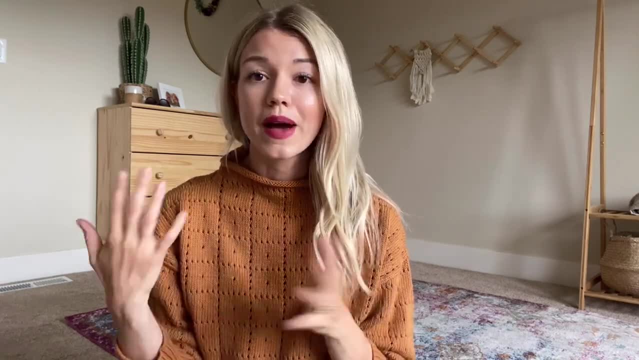 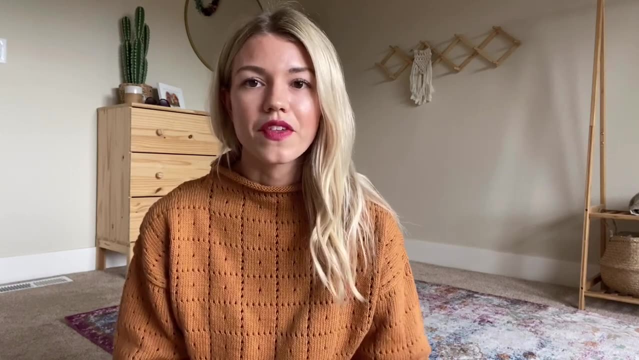 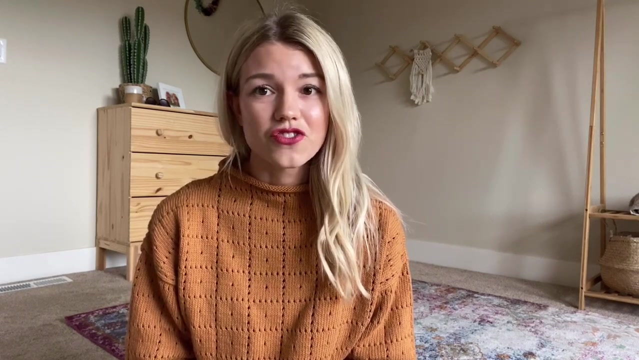 And then, um, we also- uh, our backyard doesn't really lend itself to like building a garden space, Um, so I knew right off the bat that I would need to do container gardening. Um, and that kind of seemed daunting for me because I don't know anything about gardening in general. 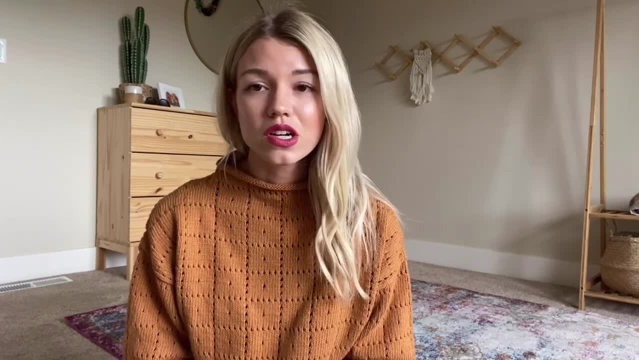 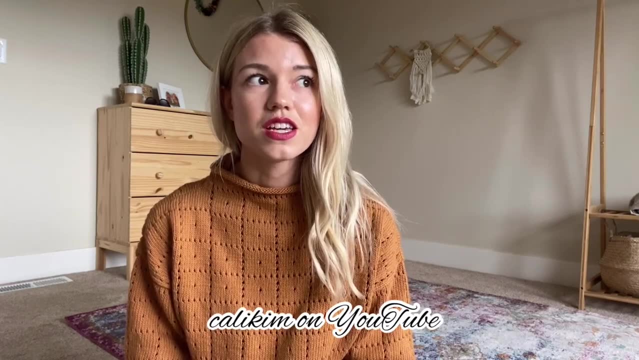 And gardening containers seemed really scary. So I just started researching Um and I started by watching some videos on YouTube And Callie Kim- she's amazing. She is the one that kind of um helped me realize that container gardening didn't have to be that hard. Um she introduced 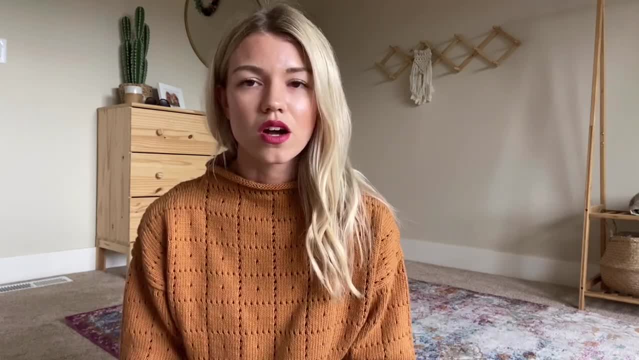 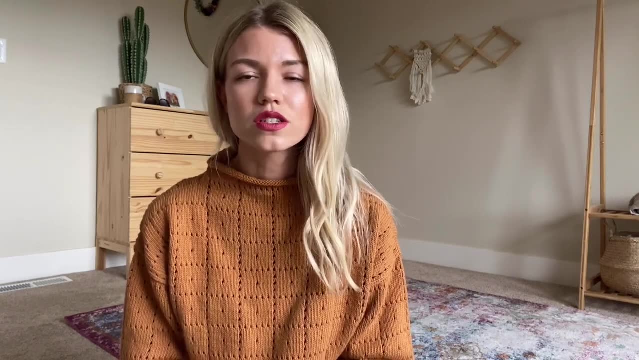 me to all of the supplies that I ended up using. I love how she makes gardening accessible. I listened to a few podcasts where I'm like, okay, this is way over my head Talking about fertilization and just germinating and things that I wasn't able to realize, And I was like 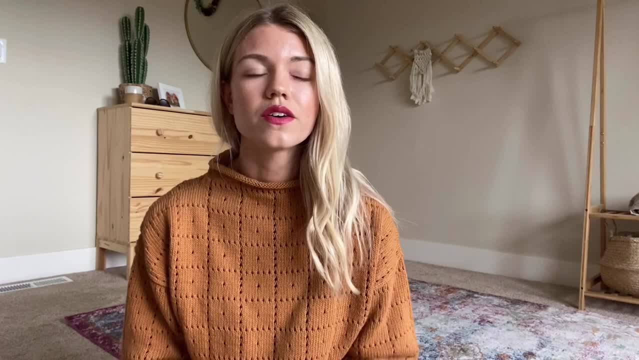 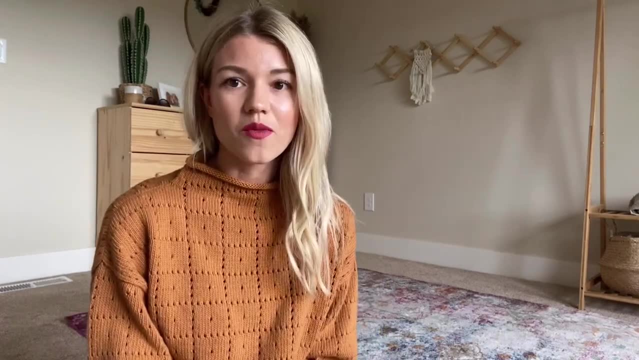 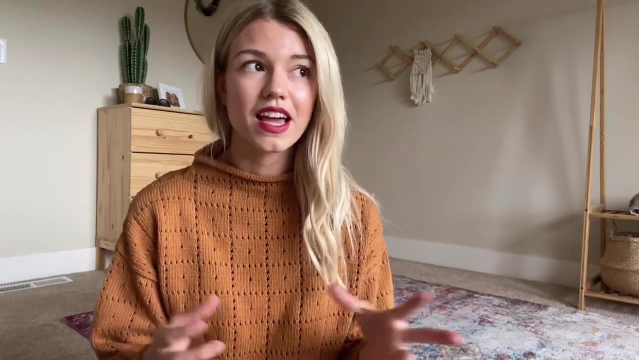 this is what I really grasp as a total beginner gardener. Um, and I also wanted this to be really kid centered and, like kid friendly because, um, my daughter wanted to be part of it. We ended up um gardening in three 20 gallon smart pots And since then I've kind of expanded how much I'm. 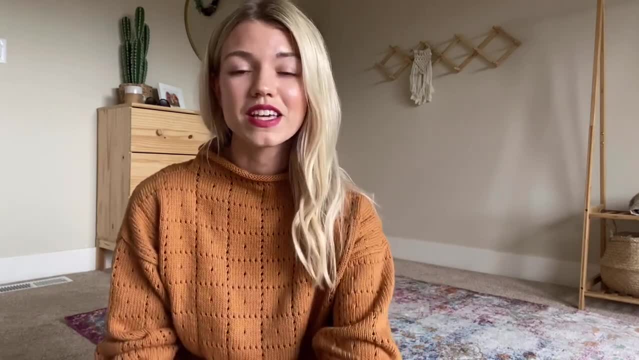 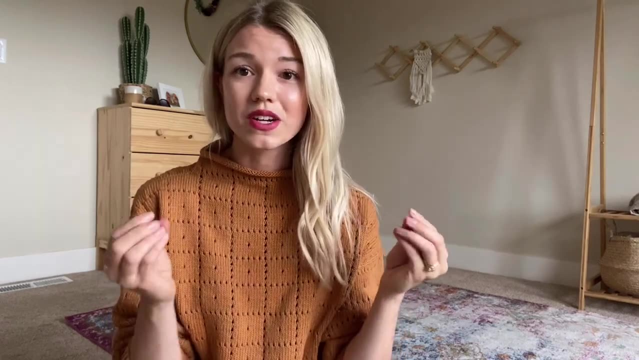 going to grow And, um, I but because I'm loving it. but yeah, we started off with three 20 gallon aerated containers, So they're kind of, they're a fabric It feels like felt And it's quite. 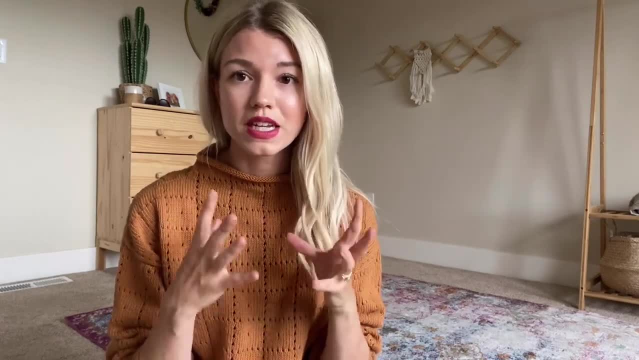 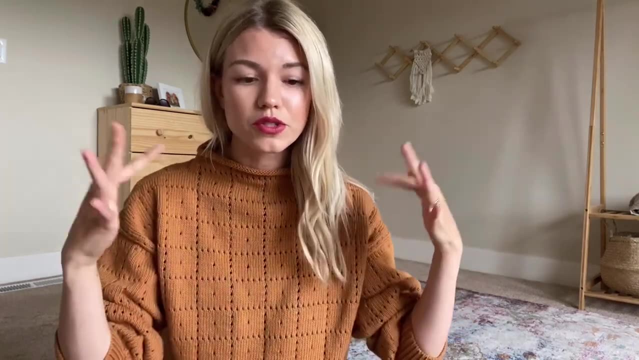 fascinating because I guess it helps the root ball form in a different way and it doesn't really grow at the bottom. It kind of is able to expand and there's more moisture that's able to go through them. So yeah, they're supposed to be really amazing. So far I've had a really 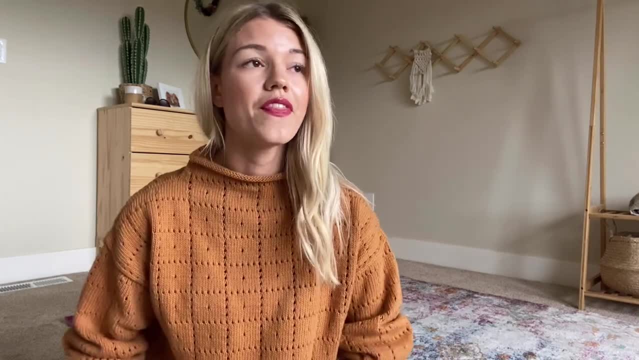 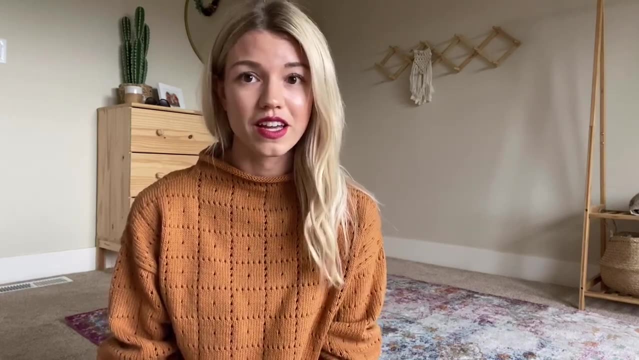 really great experience using SmartPots. And then I partnered with Good Dirt. They are not sponsoring this, but they did provide lots of product for me to try out- gardening Kind of bounced ideas off of them and they were a really great resource for me too. So in addition to 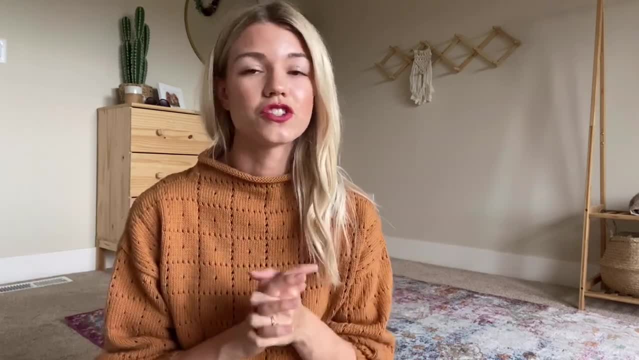 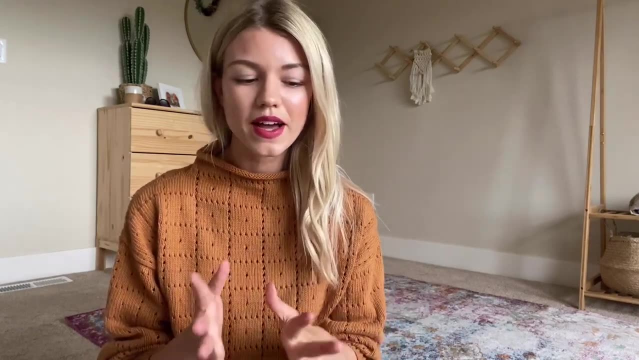 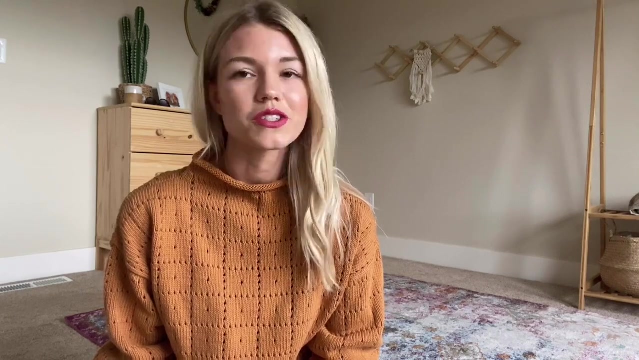 podcasts, YouTube and a couple of books. Good Dirt was a really good resource and their soil ended up being really great. I have been let's see three weeks now. I have had my plants for three weeks and they're thriving. It's so exciting and so rewarding to see how well they're doing. 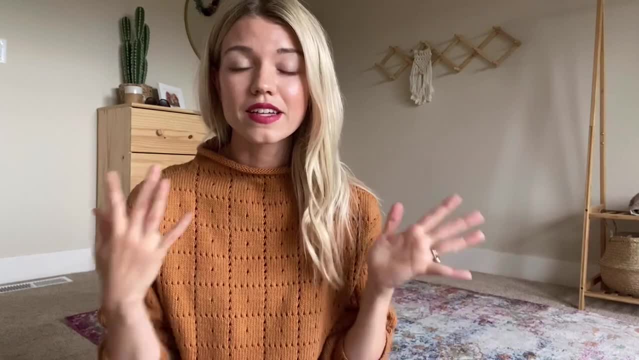 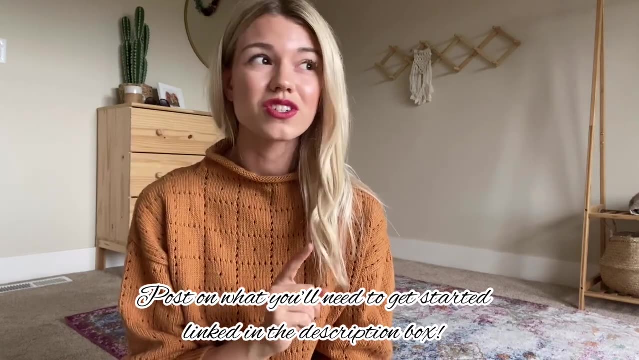 They have new growth on them. So anyway, I stocked up on my supplies and I'm not going to go through that in the video, because I have a post on my website where I listed off all the things I bought, which it wasn't that many. 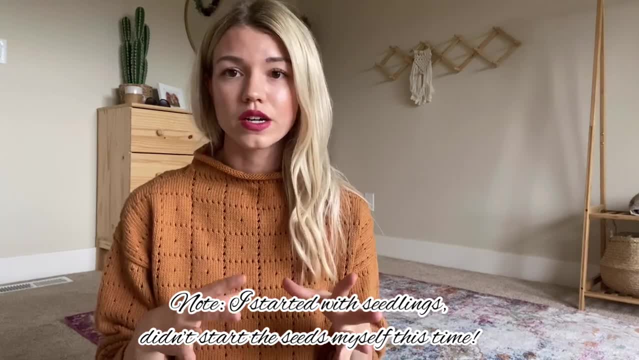 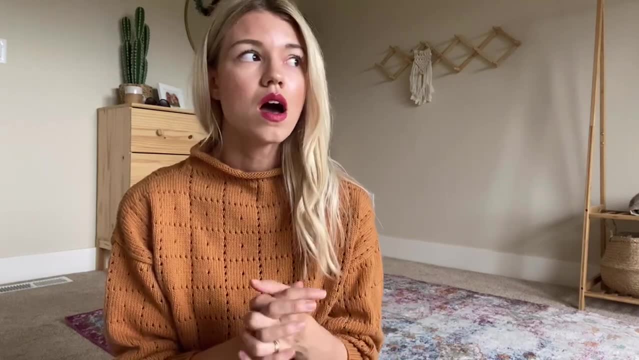 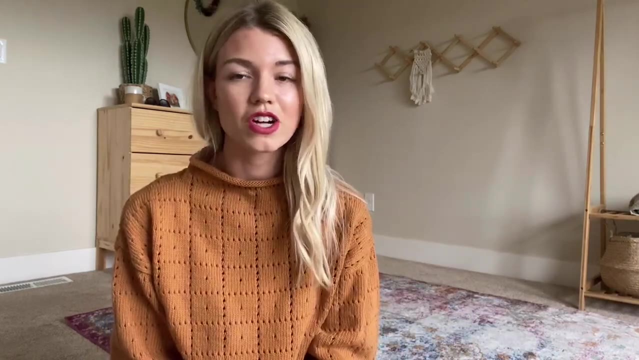 things. So I actually started our garden with seedlings. I bought them. I bought organic seedlings at our local grocery store. It's really nice that they have those. But yeah, so I did that. I did not grow from the seed this year. I might try that next year, but I wanted to start with. 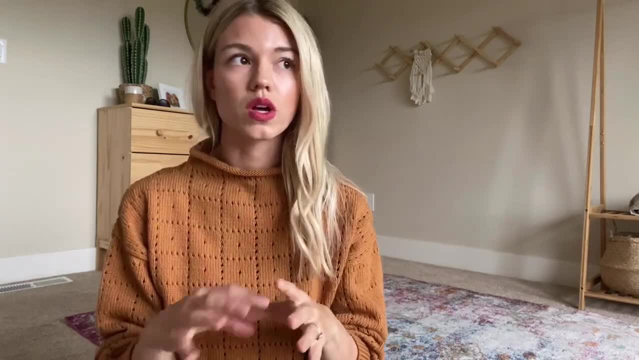 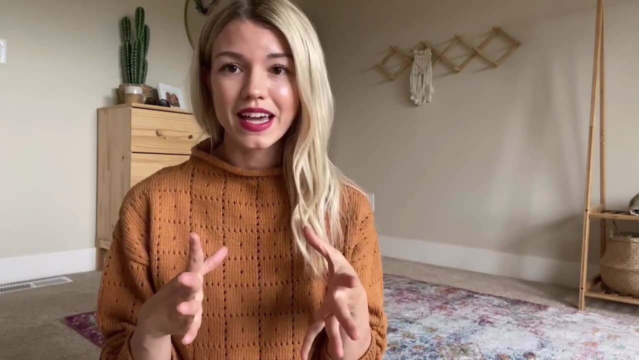 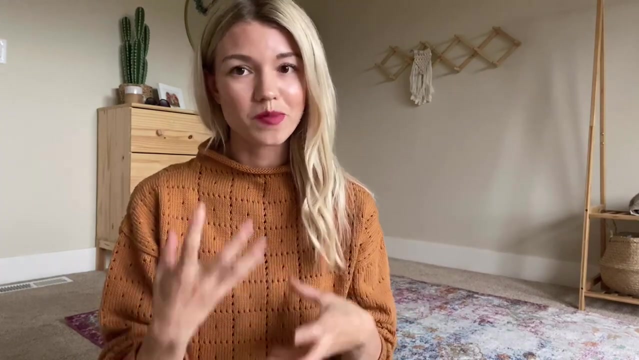 the seedling And then just plant them into the soil and just see how they thrive and just kind of try my hand at it that way first. So anyway, I gathered my supplies and then I actually filmed myself with my daughter planting our third container, or planting our third container of plants. 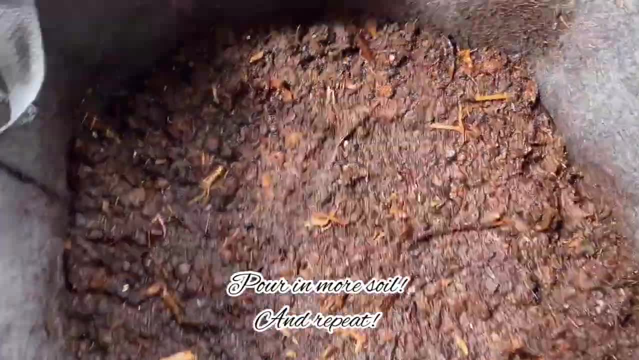 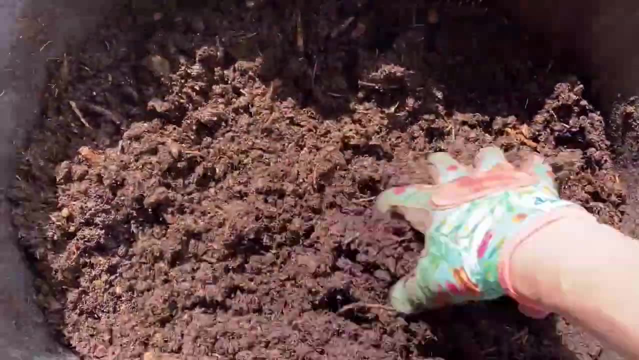 So that's how we started, And my daughter's starting to like our new garden. I'm going to show you pick some of the flowers and then we're going to see how we grow them And then I'm going to show you how we do the flowering of the flowering. 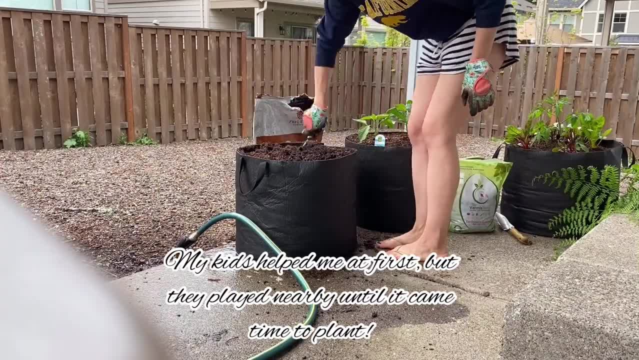 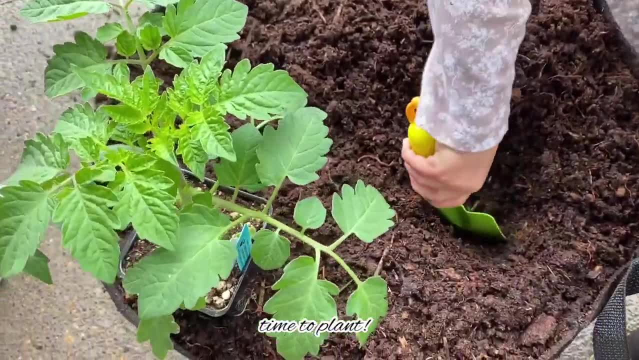 So the first thing I'm going to grow is a six foot flower, And the first thing you're going to do is you're going to take your seedlings. So you're going to take your seedlings And you're going to have a very nice little flower. 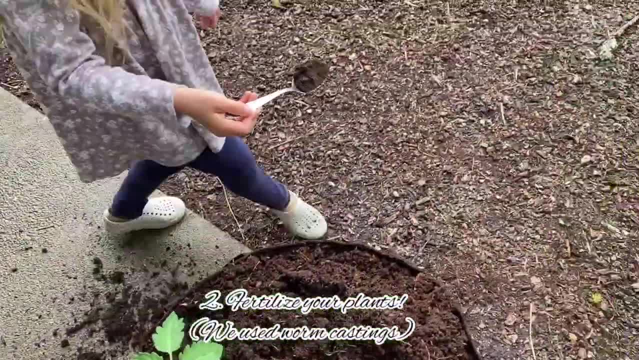 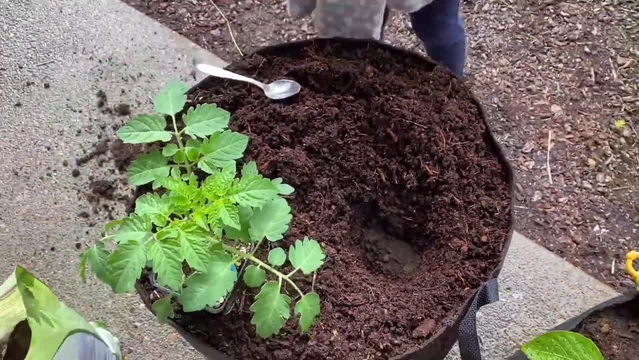 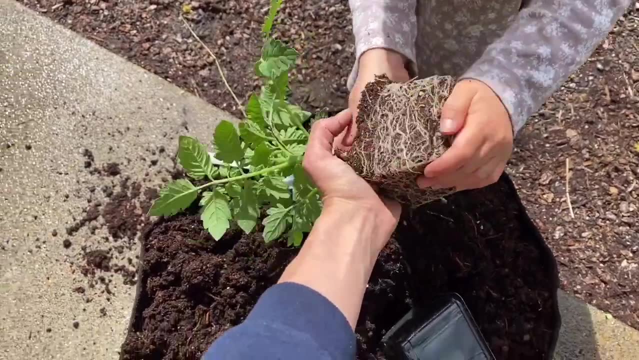 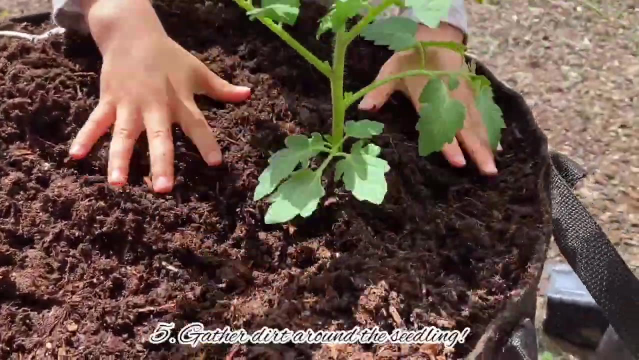 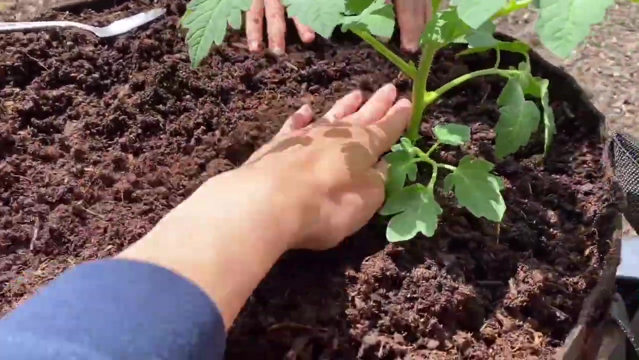 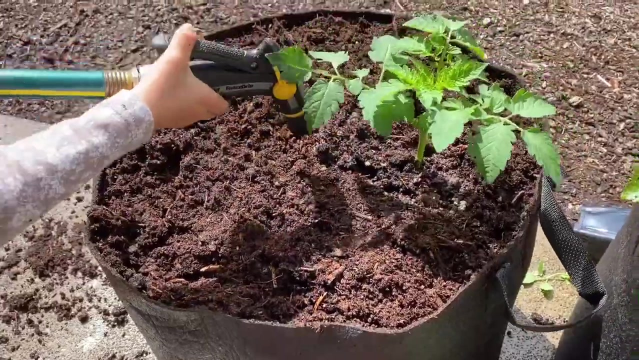 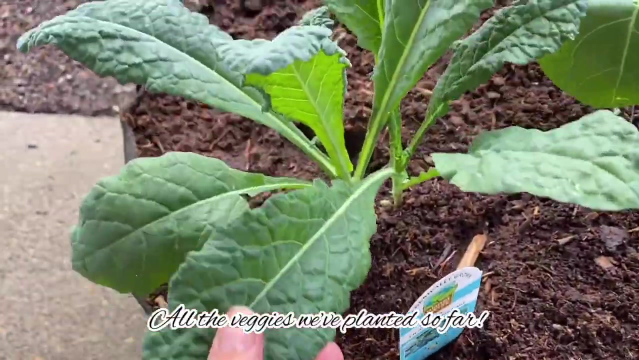 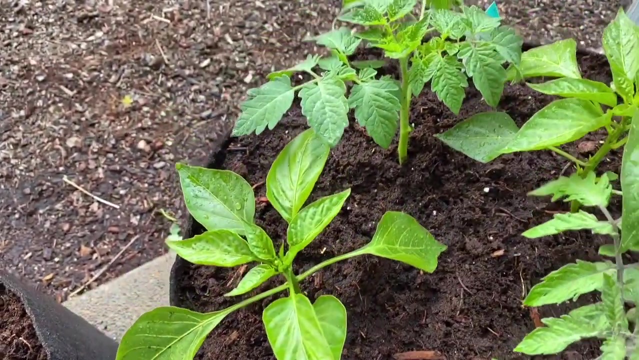 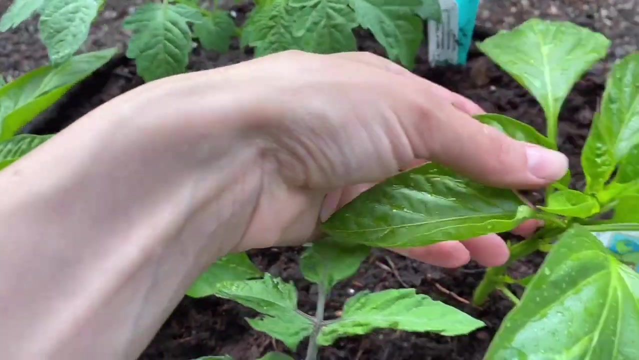 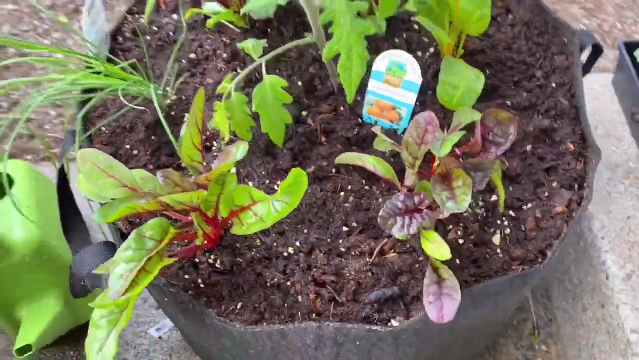 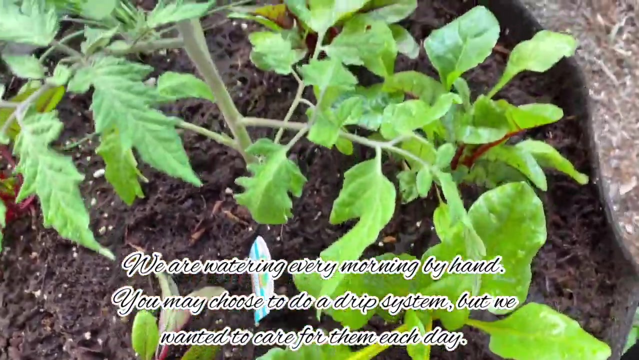 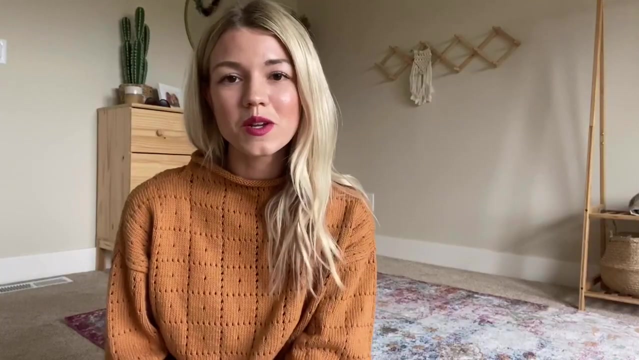 So I'm going to do that. So this is what they look like. These are the flowers, These are the seedlings, These are the plants. Thank you, Thank you. Like I said, it's been a really rewarding experience. My daughter has had such a good time watering our plants every day.